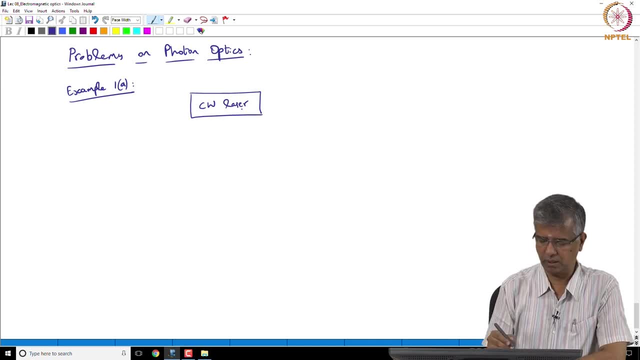 So you are told that this continuous wave laser has a wavelength of 0.2 microns and it is emitting radiation which corresponds to 1 nanowatt of power. ok, Now what you are asked to figure out is: if you, if you put a detector over here, then what? 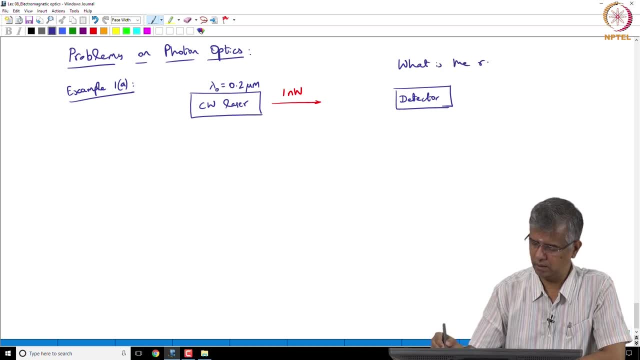 is the rate at which photons fall out of the atmosphere. Ok, On the detector. So what is the rate at which photons fall on the detector is what you are, you are, asked to figure out. So what we see is in conventional wave optics, you deal. 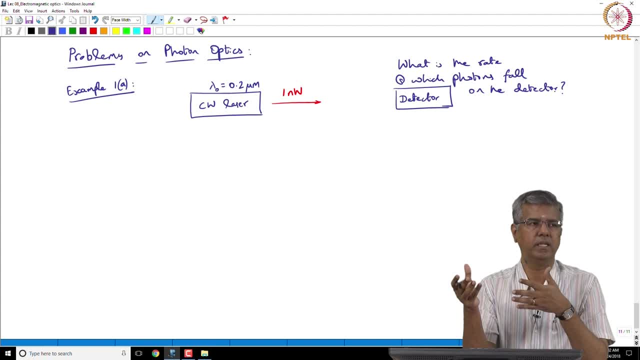 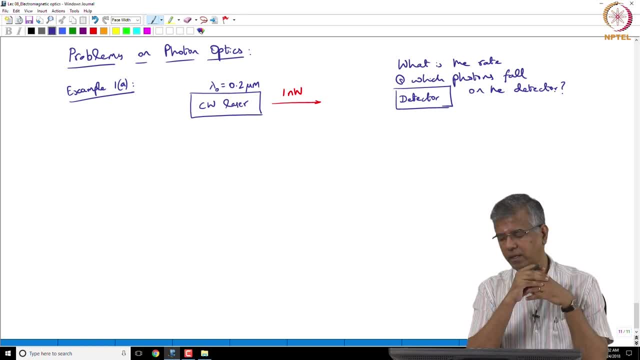 what is the rate at which photons are arriving at a particular point. So that is, that is what we call as photon flux. What is the photon flux density? ok, per unit area. what is the photon flux density? and then what is the photon frequency? So what is the current density? 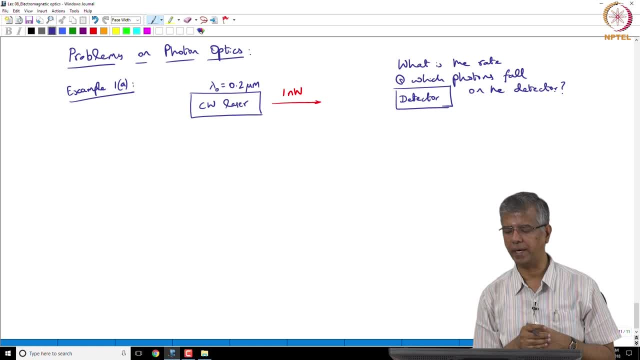 of the photon that we get at a particular point. So those are the quantities that we will start looking at. ok, So for example, here, what you are asked is the photon flux. So photon phi is going to be given by the mean number of photons falling on the detector per unit. 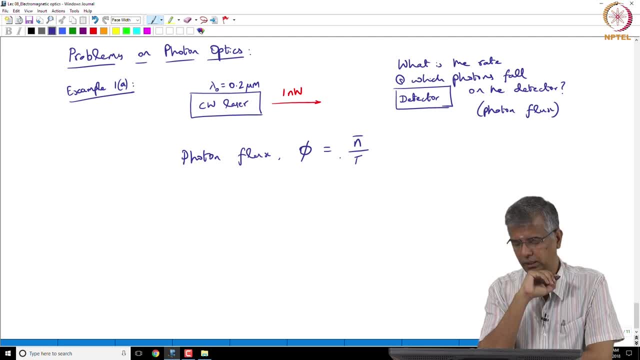 time. ok, So n bar here corresponds to mean number of photons, right? So what is n bar? If you know the energy of light? ok, Can we find what is the mean number of photons? So mean number of photons n bar. how is it? 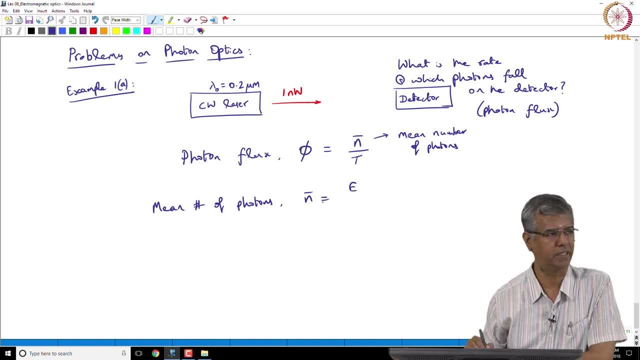 related to the energy. if your energy of your radiation is E or divided by h, nu, which is the Energy corresponding to a single photon, right? So now we can. if you are given power or energy, you can actually figure out that in terms of number of photons. ok, And of course I. 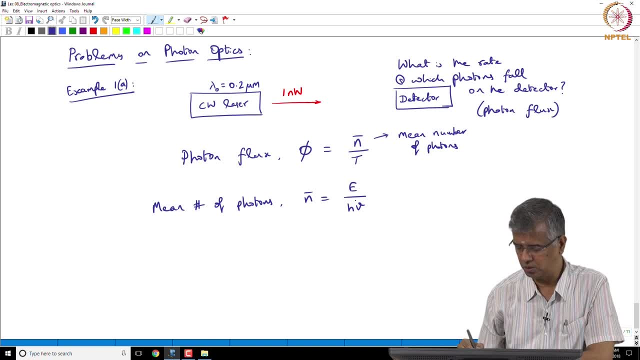 say h nu, I may also use h nu bar. where would I use that If I have a? if I am given a broadband source, right like what we were looking at yesterday, your source has got multiple frequencies in it and then you have a central frequency. 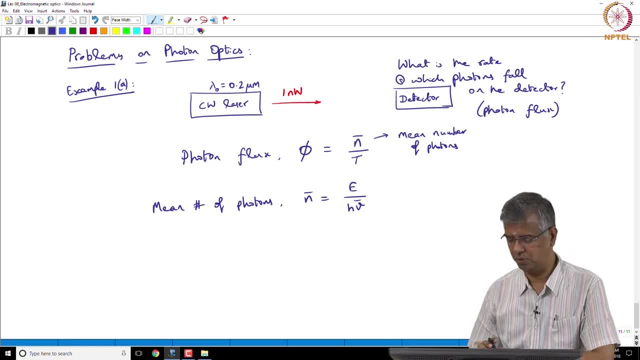 right that centre frequency you may take as mu bar. ok, So in this case you are given power right. given optical power, how do you convert energy to power? what is the relationship? zwei times the power integrated over time is energy right. So P times T divided by h, nu. and so now, 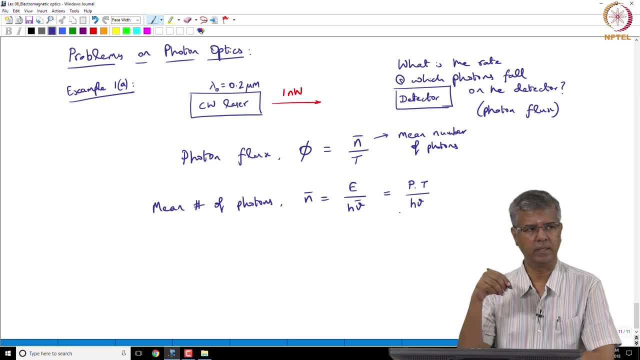 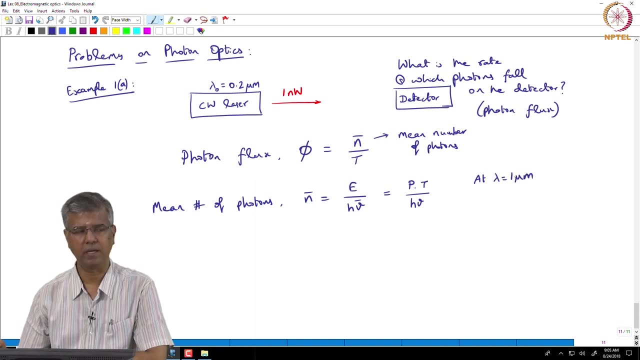 we need to find out h nu for the given laser. the laser is oscillating with 0.2 micron wavelength right? So we know that at lambda equal to 1 micron, what is the corresponding E? What did we see? 1.24 electron volt, right. So you are asked to figure out the. 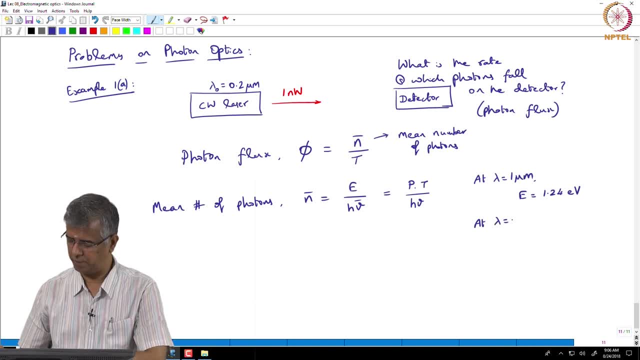 energy of a photon at lambda equal to 0.2 micron. what would this energy be? So it is 5 times lower wavelength, so the energy should be 5 times higher, right? So 5 times 1.24, that would correspond to 6.2 electron volt, right? So? 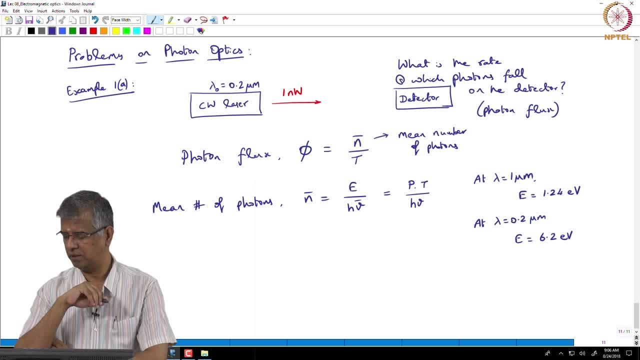 lambda at 0.2 micron is 6.2 electron volt. and if you convert that into joules, what do you multiply that with 6.2, multiplied by 1.6, into 10 power minus 19 charge of an electron, and that 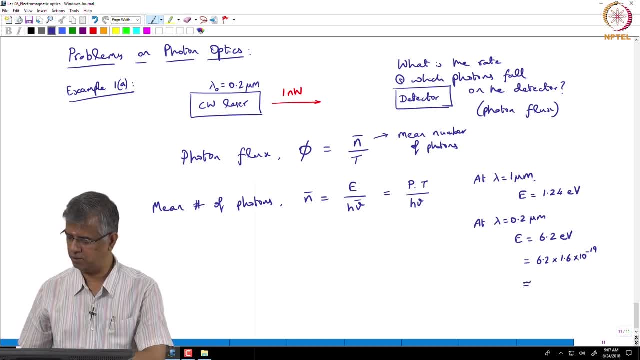 would give roughly 1.6 into 10 power minus 19 charge of an electron and that would give roughly about 6.2 and 1.6 would be roughly about 10, so that is about 10 power minus 18 joules right. 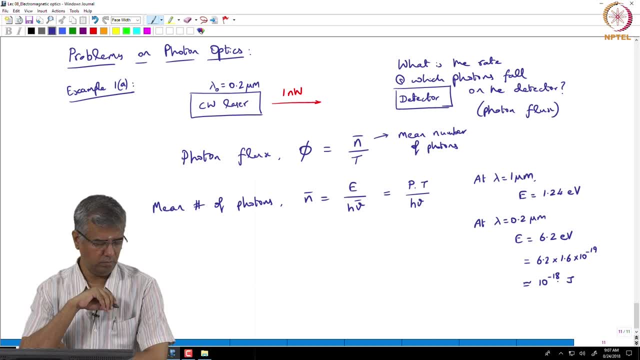 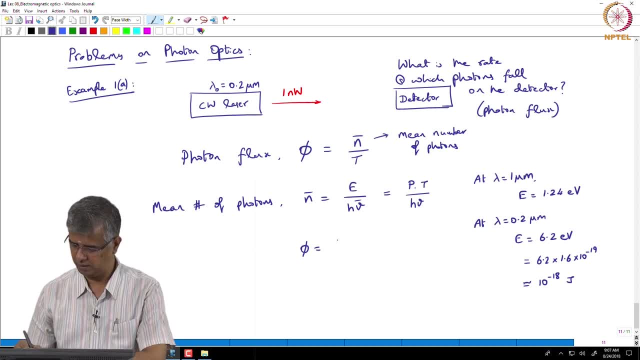 so I substitute this expression. so I substitute this expression. So then what you get is essentially that the T in the numerator and denominator will cancel each other. so what you get is: this is going to be equal to the power divided by H. nu. ok, Since I am having 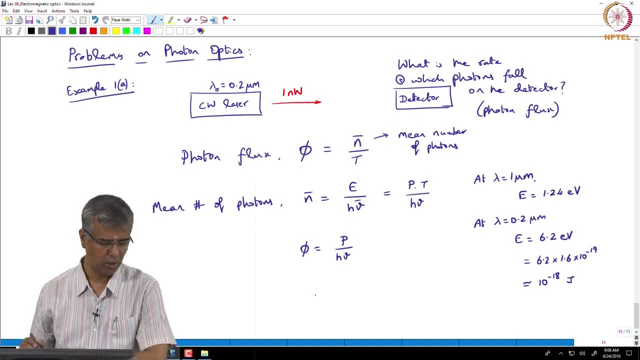 only one wavelength given. I can just take it as H nu. so this is so. the power that is given is 10 power, 9 right 1 nanowatt and h nu we have figured as 10 power minus 18. ok, So that corresponds. 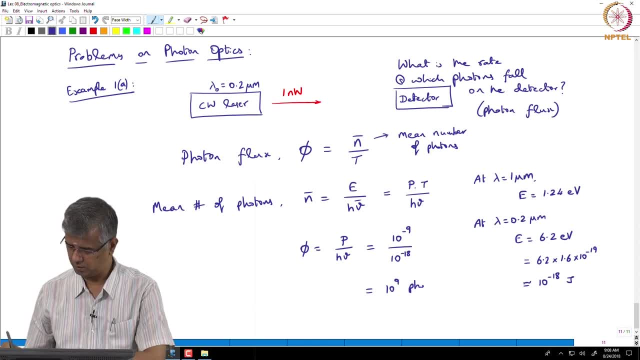 to 10 power 9 photons per second right. So the photon flux is 10 power 9 photons per second, which is corresponding to the power of 1 nanowatt at a wavelength of 0.2 microns. So this is actually. you can also say that this means that I have 1 photon arriving per 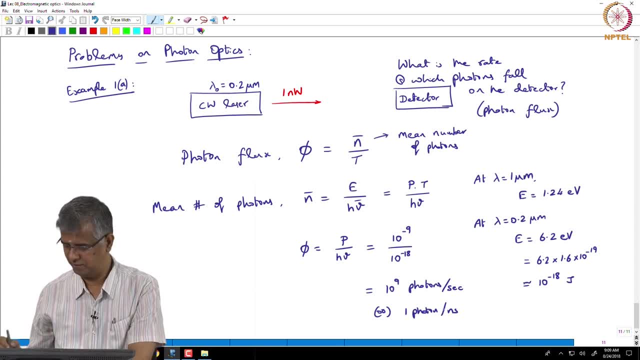 nanosecond right 1 photon arriving per nanosecond on the average. So this would be an interesting experiment. I was hoping I could give you a demo of this. we have done this before, So you take a laser and you know you take maybe. 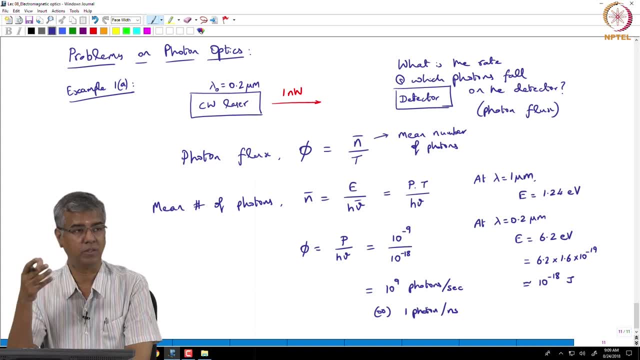 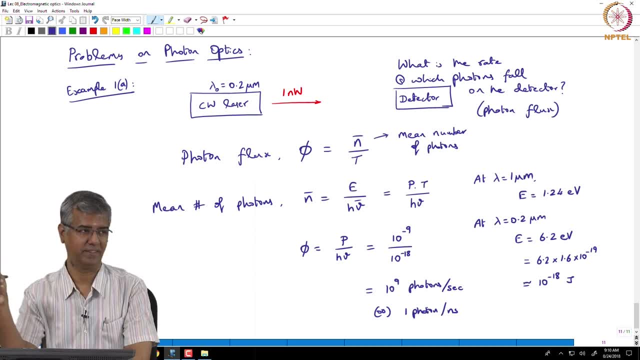 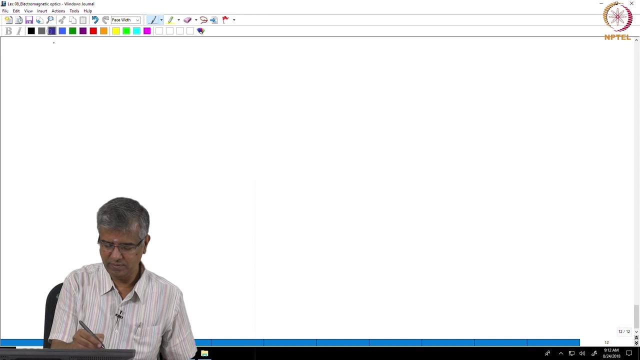 in number of photons and photon density and so on. So let us move on to another example, Example 1B. let us say- and this is actually related to something called laser assisted- 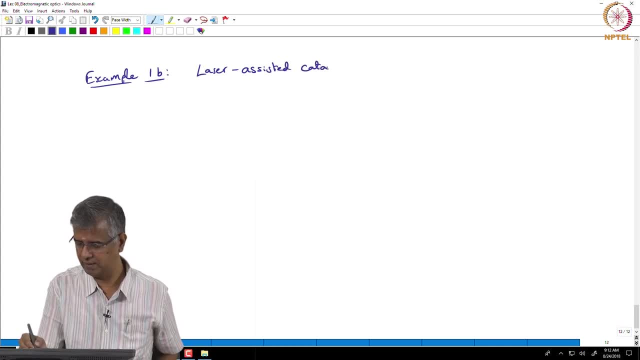 cataract surgery. So you know, we have actually started a company that makes fiber lasers. you do not know what a fiber laser is- maybe I will come back and talk about that later on- but we make fiber lasers and we make pulsed fiber lasers, and these fiber lasers are: 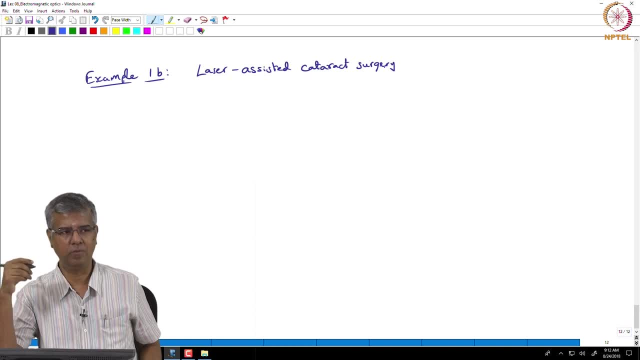 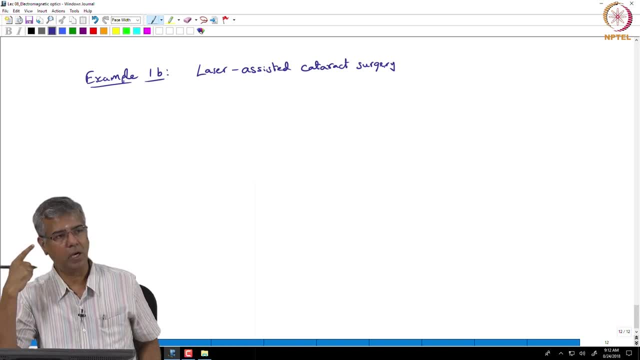 whether this laser can be used to ablate tissue in the eye. ok, So that you can. you can basically make a very precise incision in one of the tissue layers in the eye and you can, through that you can do cataract surgery. ok, So that is what laser assisted. 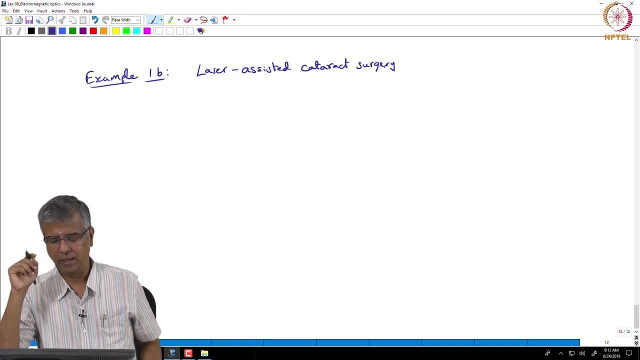 surgery is. So that is what laser assisted surgery is. So that is what laser assisted cataract surgery is all about, and in this case, we use a pulse laser. ok, So the pulse laser. you know it is emitting pulse laser, emitting 100 femtosecond pulses. 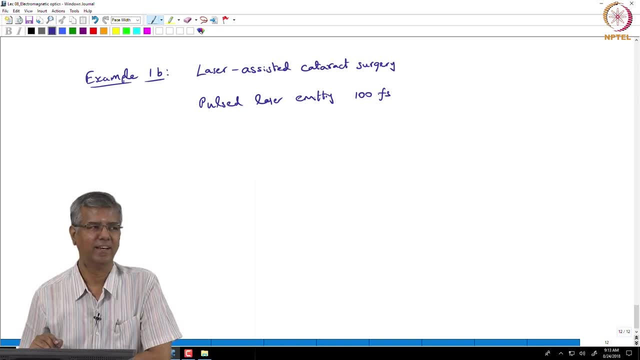 what is the femtosecond? 10 power minus 15 seconds, right? So it is pico, which is 10 power minus 12.. So 0.75.. So 0 Pico, which is 100 femtosecond. 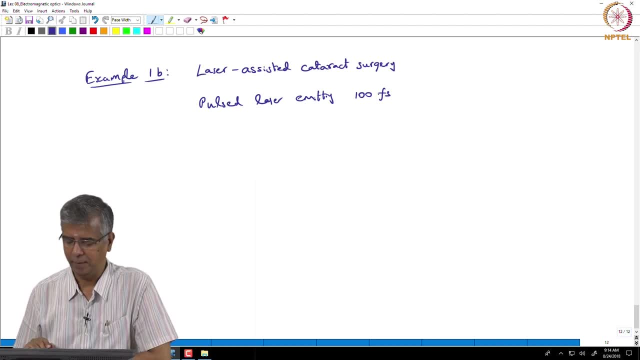 So 0.75.. So 0.75.. femtosecond pulses at wavelength of 1.06 microns. why that specific wavelength? we will come back and look at that later, when we discussing lasers. but let us say this is emitting these pulses at 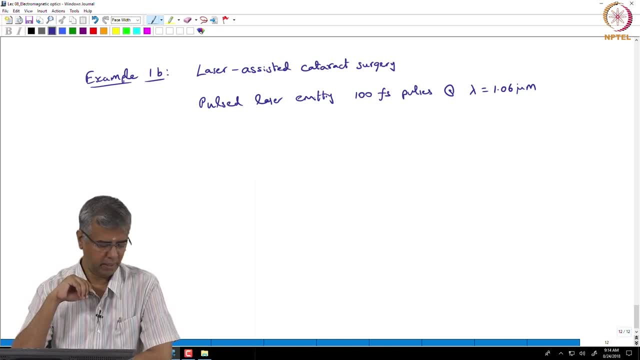 1.06 microns and you are told that you need 1 joule per centimeter square energy density to create, to basically punch a hole through the tissue layer. So this is a process that is called photodisruption that you are doing, where you are actually cutting tissue with these pulse lasers. 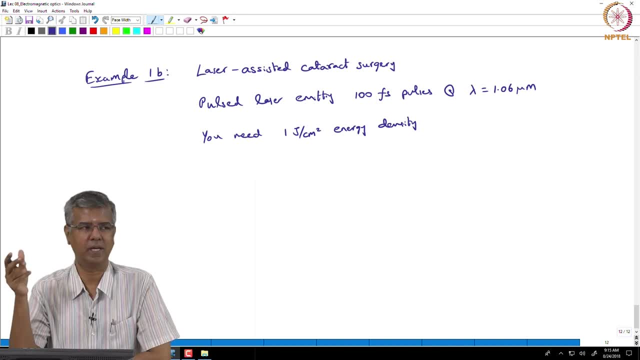 And why do you so? you can always use a high power laser and cut tissue, So why do you want to use a very short pulse laser? any idea? If you are continuously depositing energy on the tissue, it will be absorbed by the tissue, and then there is a 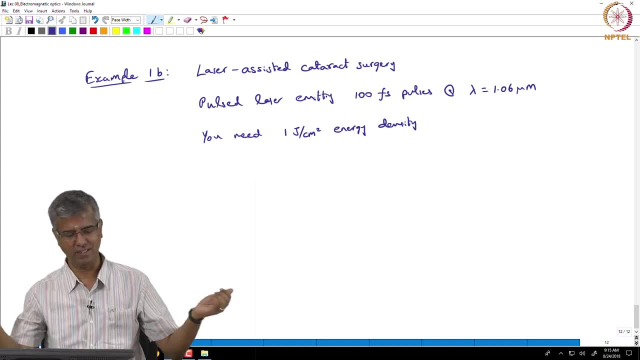 heat dissipation. So this is called photodisruption. So if you are continuously depositing energy on the tissue, it will be absorbed by the tissue and then there is a heat that is generated. That heat will, you know, spread around the tissue and it will end up charring the 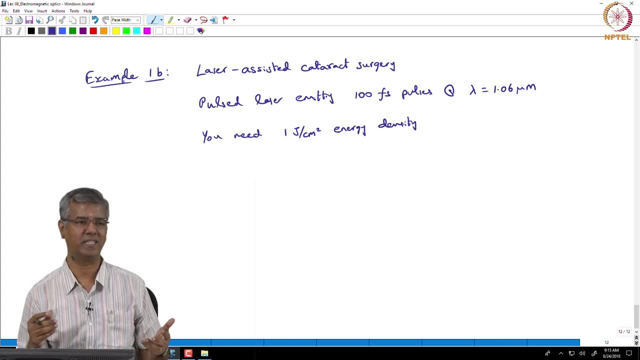 neighboring tissues. also, There will be a lot of collateral damage. that is happening. But if you are using 100 femtosecond pulses, what are you doing? You are packing a whole lot of photons within a very, very small duration. So it goes and hits and it does the work of 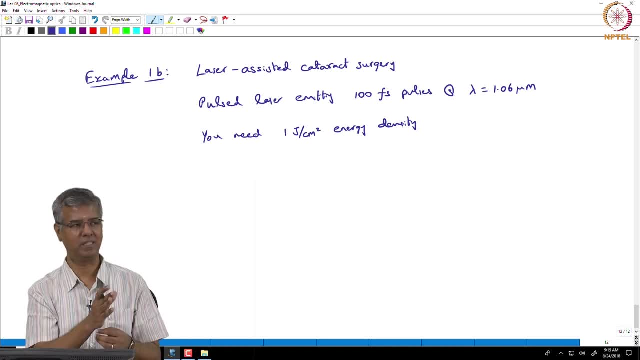 you know, getting absorbed and then it is rupturing the tissue. But since it is all happening within that 100 femtosecond time scale, it does not. the heat actually builds up over millisecond time scales. So if you are doing much, much shorter than that, there is very 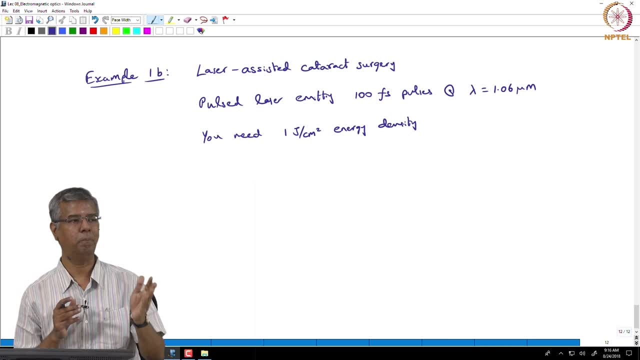 little collateral damage that is happening, So you can get very precise cuts if you are using such short pulses. ok, But but you need you are told that you need 1 joule per centimeter square energy density. So the question is, what is the corresponding photon flux density? ok, So that is what you. 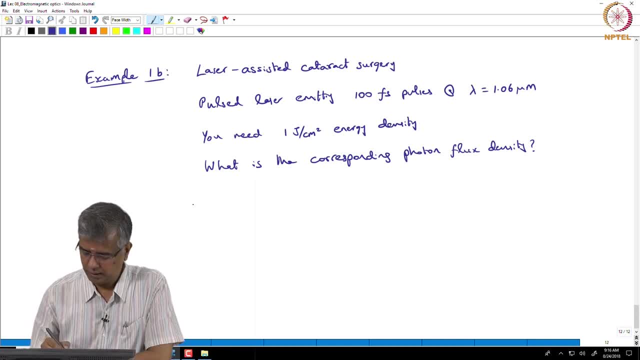 are you are asked to figure out, And photon flux density, what do you think that that corresponds to at a particular location, Let us say it is a small phi of r would be what Would be photon flux per unit area. ok, So that is what you are asked to figure out. So that is what you are asked to. 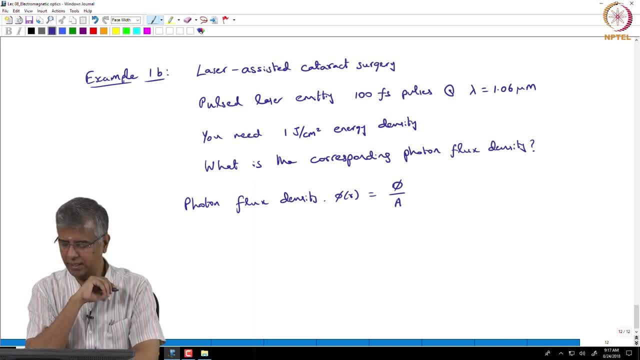 figure out right. So that is what photon flux density is, and we know that from our discussion in the previous problem. we know that phi corresponds to n bar over t. ok, So you can, you can substitute that over here, and what you are given is actually mu dot boys. 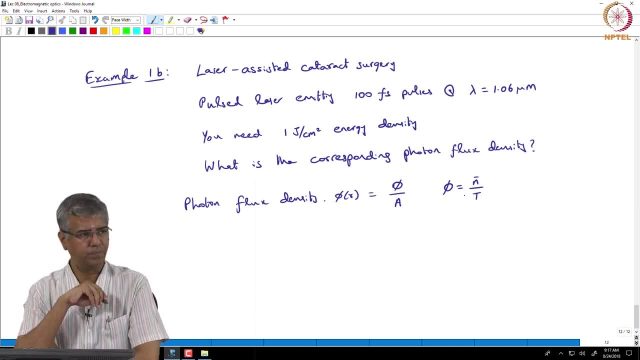 Now if we was actually down a break two 떨 쩐 30 Ты Hu T East Z am ve o 2 t 19, 0, 20 warm 10, 18, 20 energy density. right, So you can basically say this is going to be equal to n bar over. 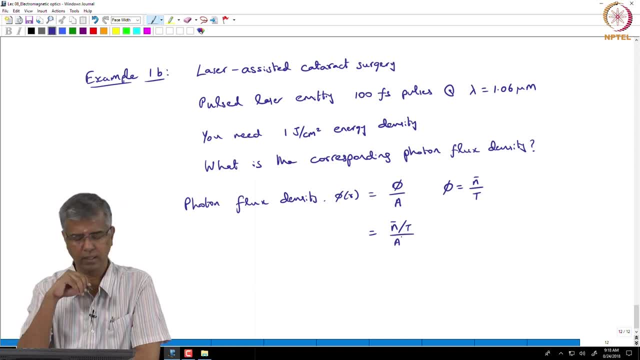 T over A right, but n bar over A. So I will keep 1 over T outside right and n bar over A can be expressed: n bar is, in other words is basically E over h nu right, So you can write this as E over A times. 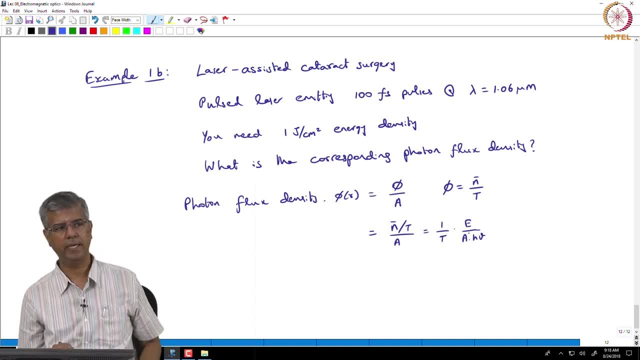 h nu right. and what are you given? You are given energy density, which is E over A right, And so if you substitute that, and then you can actually, and you are all you also given this time. So based on that, you can figure out. So let us just, first of all, 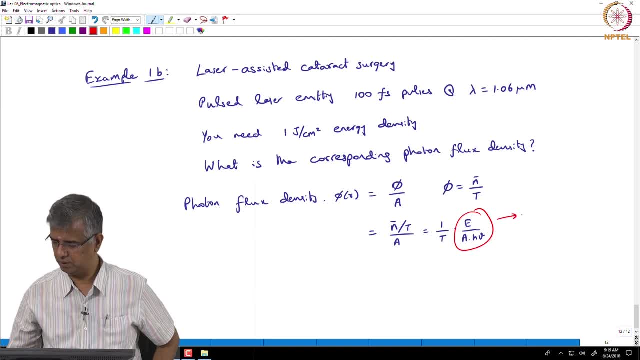 figure out this quantity. So this is given by E over A, which is 1 Joule per centimeter square divided by h nu, h nu for a lambda of 1.06 micron. what do you think would be? Let us put around something around 1.24, and all right. 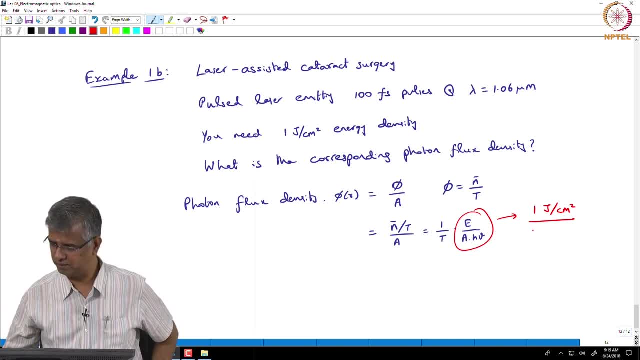 electron volt, right, So this is basically 1.24 electron volt, and then you convert that to joules, right? What do you do? Multiply by 1.6 into 10, power minus 19,, right, So? 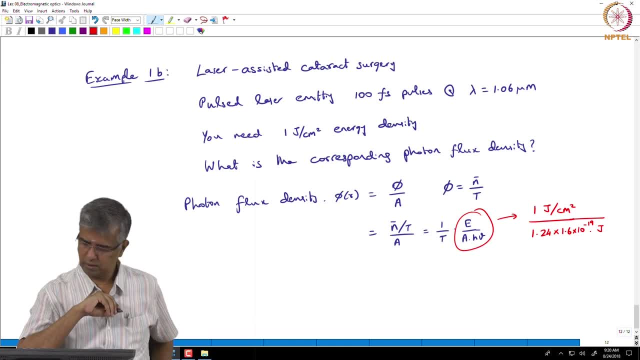 that will be in joules, right. So if you do the math, you will probably get something in the order of 5, 0.5 into 10 power 19, and this will be in terms of photons per centimeter square, right. So that will be the quantity here. and to get the photon flux density you 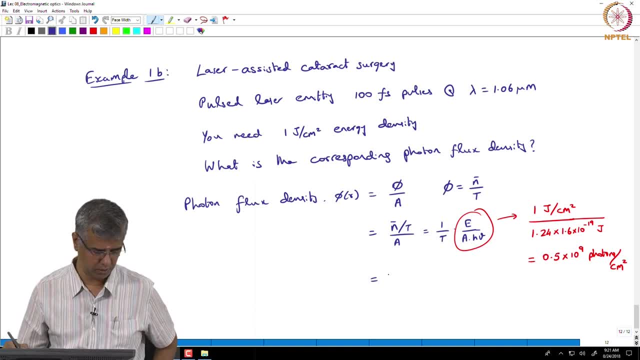 just substitute that into this other expression, which is basically: you say 0.5 into 10 power 19 over the time. the interaction time here is 100 femtoseconds, right? So 100 into 10 power 19. businessmanelectron full-time Babier. 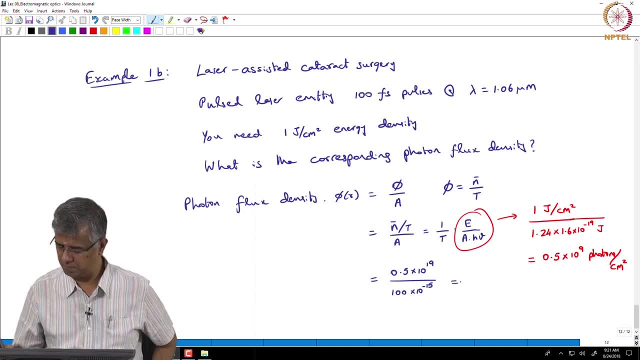 minus 15.. So if you do the math, that will come out to be about 0.5 into 10 power: 32 photons per second centimeter square. so that is the photon flux density that you need. Now that is actually sounds like a really large number, but you know what probably makes sense. 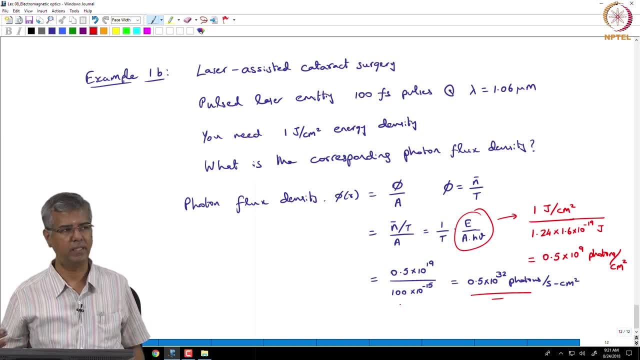 is that it is not the photon flux density that you are interested in. you are looking at the photon density, So you are actually. you already packed so many photons. how many photons are you packing? You know something? the order of 10 power. I put it as: 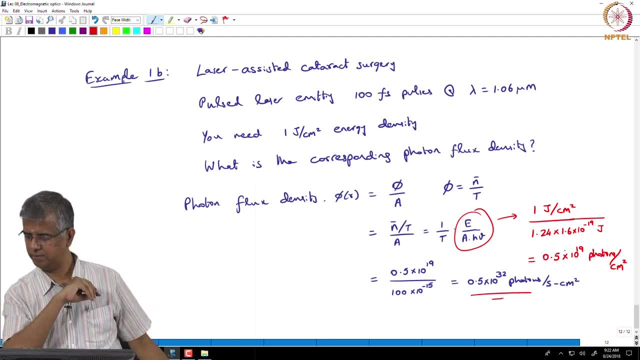 it should be 19 here, right? So that is 10 power, 19 photons per centimeter square. but you are not doing a hole over a centimeter square area, right? that will essentially take out your eye completely. So you are actually doing holes, some micron holes, right? So when you do, 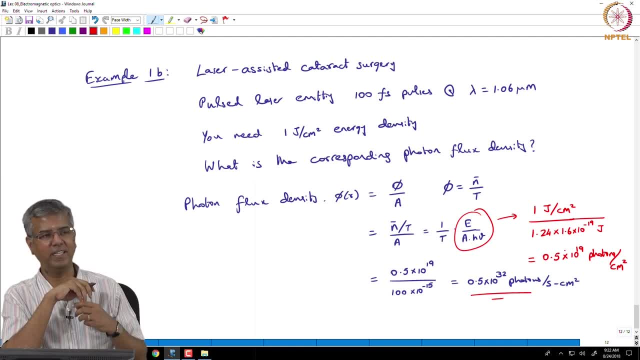 it in terms of micron square? right it is. it may be 100 micron square, so the number of photons is in the order of 10 power, 12 photons, but that is still a huge number. you are talking about a trillion, so million, billion, trillion, a trillion photons. right, you are packing within. one pulse, one bullet. 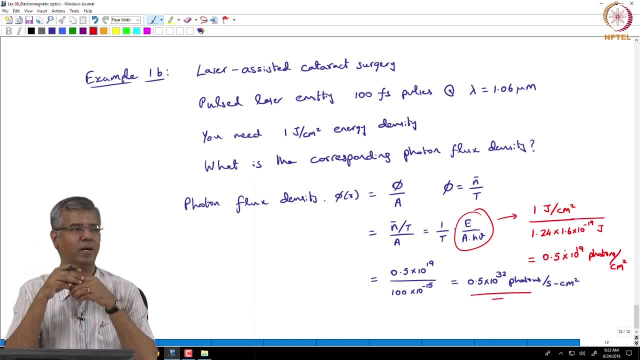 And you may actually require multiple pulses to do the precise cutting. so you are like it is like a machine gun. it is just hitting with bullets, and these bullets are extremely powerful. I mean, you are talking about packing that many photons within a very short time scale. 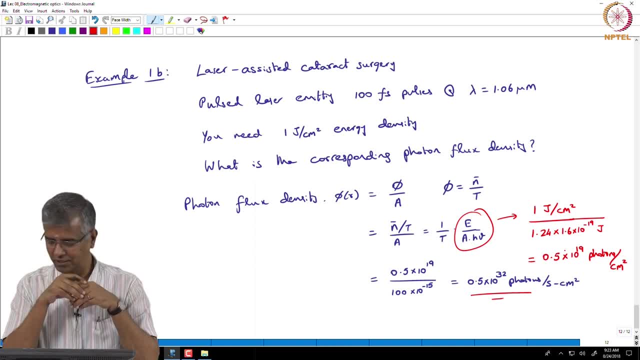 So these tissues have no chance. it will little rupture in no time. but the key point here is because it is all this interaction is happening in within a very short time scale. the thermal, you know, build up is very, very low, so you can get very precise cuts. 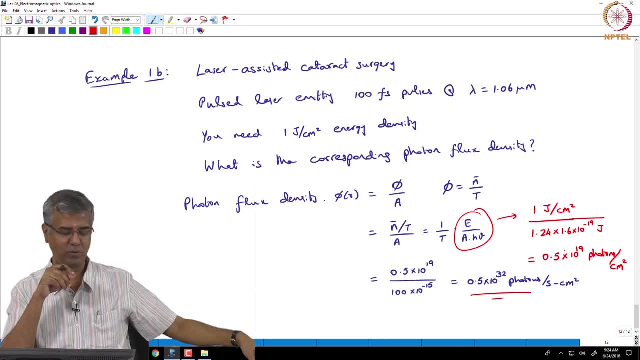 Now it could be your eye, it could be this wooden table here, it could be, you know, a metallic part where you want to make a very precise incision. you want to actually do some patterns in a metal, some micro machining that you want to do in a metal. all of that you can do if you have. 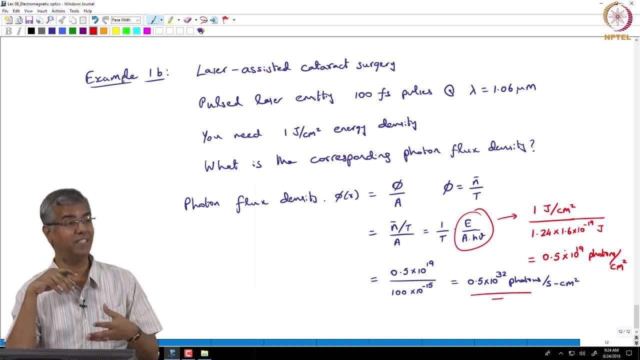 femtosecond pulses. ok, How we generate these femtosecond pulses, we will have to wait. I mean, there is still several weeks away. we will come back and look at that little more detail, but if you have a such a source, you know this is what you are dealing with. I am just trying. 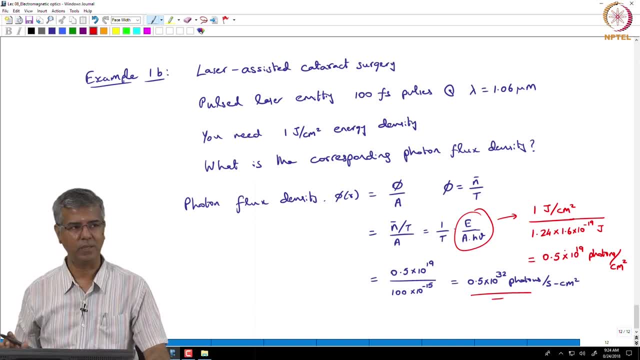 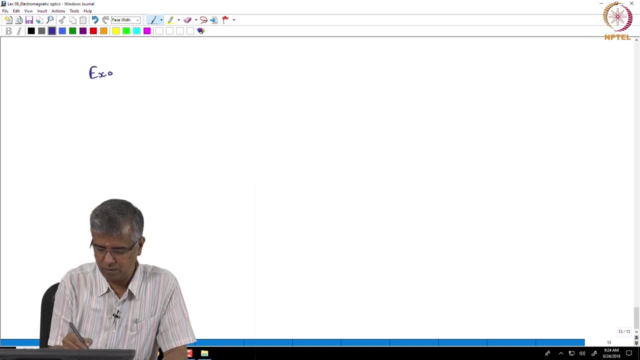 to give you a picture in terms of photons. Any questions before we move on? Ok, Ok, Ok, Ok, Ok, Ok. Let us now look at another interesting example, example 2, where we are looking at optical communication. right, So in optical communication, you have basically a transmitter. 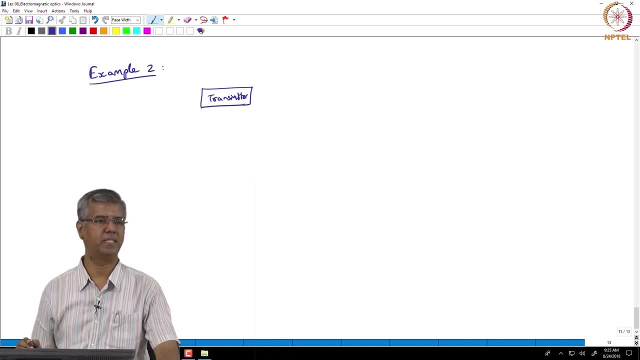 which is typically a laser based transmitter, and you are communicating information in bits, right? Let us say, you are transmitting data at 10 gigabits per second, ok, and you are transmitting in on off format. What is on off format. What is on off format On off format is: 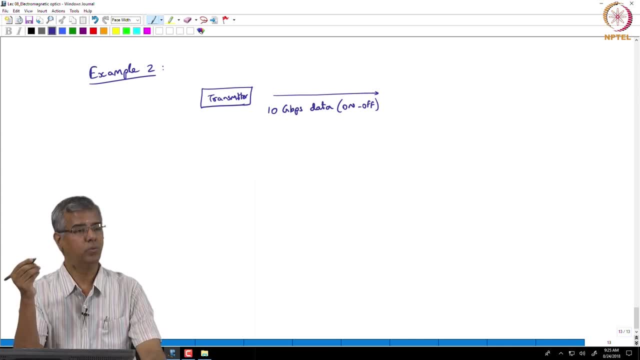 when you are transmitting data to the transmitter. So what is on off format mean One would correspond to the laser being on the, you have bunch of pulses and as a bunch of photons and off is with the laser is off right. So you should not have any photons in the in the off condition, right? So 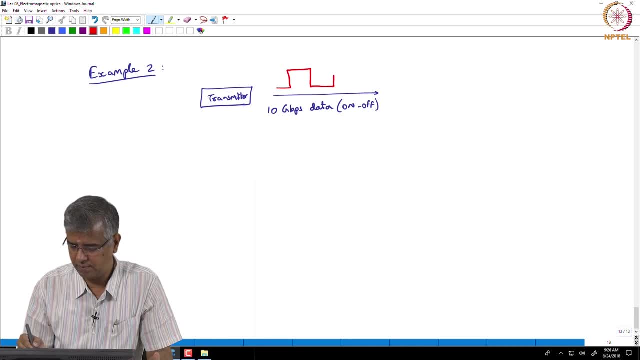 you are, you are transmitting pulses like this and if you are transmitting at 10 gigabits per second, ok, Ok, Ok, Ok, your pulse period: here the time period between two successive pulses is 1. over 10 gig. 10 gig is 10. 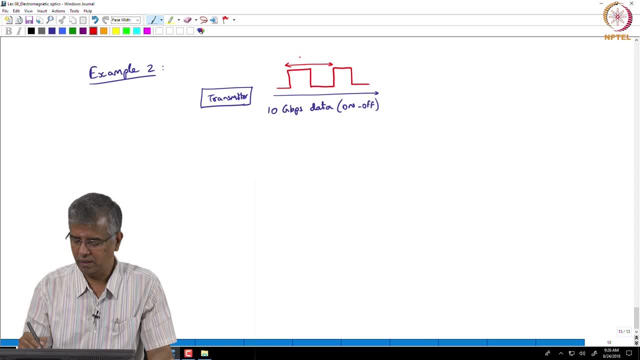 power 9, so 1 over 10 gig will be 100 picosecond. So you know, within that one bit, which is in the order of 50 picoseconds, you either turn on or turn off the photons. What you are told is, in this case: 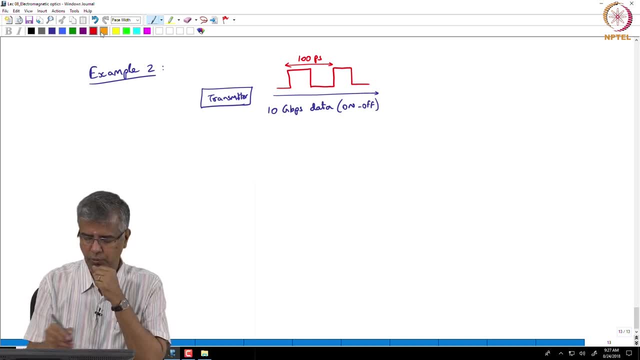 you have 20 photons. that is the mean photon. number n bar right is 20 photons and obviously with the off duration that would be 0 photons. so that is what you have transmitted and what you are asked to do is in your receiver right, what is the probability of finding 0 photons? 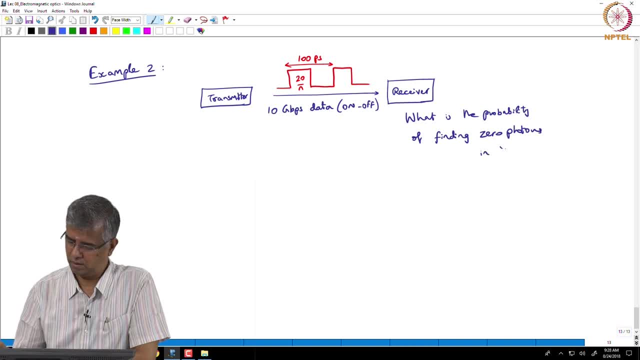 in a vacuum bit. Why are we interested in finding that? Obviously, if you detect only 0 photons in a 1 bit, then that corresponds to an error. So you want to find out what is the typical quantity by which you know you judge the performance of a communication system, a digital communication? 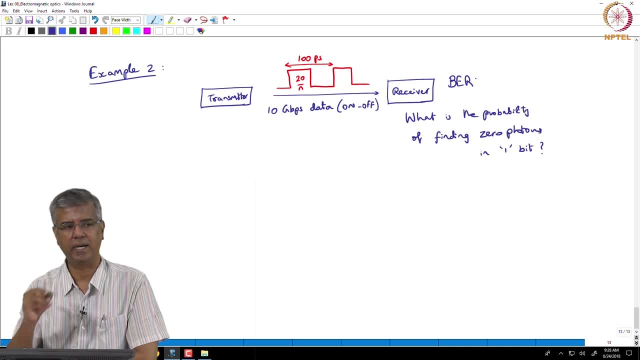 system is this quantity called BER. BER is bit error rate. So you want to look at the error rate that you are having in the communication and typical bit error rates in communication. in optical communication you try to look at 10 power minus 9. ok, So you want to achieve a BER. 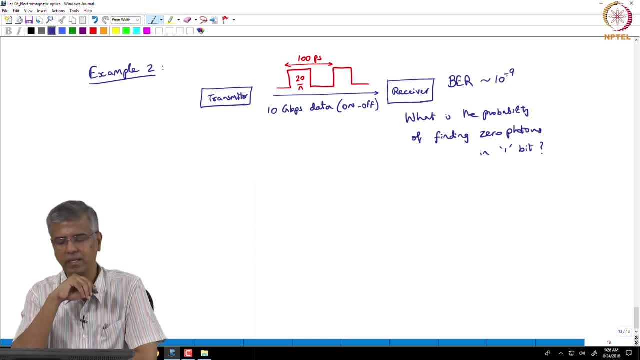 of 10 power minus 9. ok, One in a billion bit can be Trim in error, but not more than that. Did you have a question? No, ok, So we are trying to achieve that, and to achieve that you need to understand what is the probability of finding 0 bits. 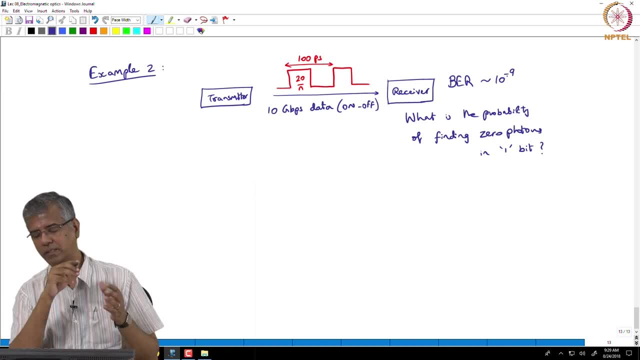 0 photons in a 1 bit. So it is given that you are transmitting a mean number. So the key point is it is this: n bar is actually a mean number of photons of 20.. What is the probability that you do not have any photons in that 1 bit at the receiver? You think, if I am sending 20 photons, 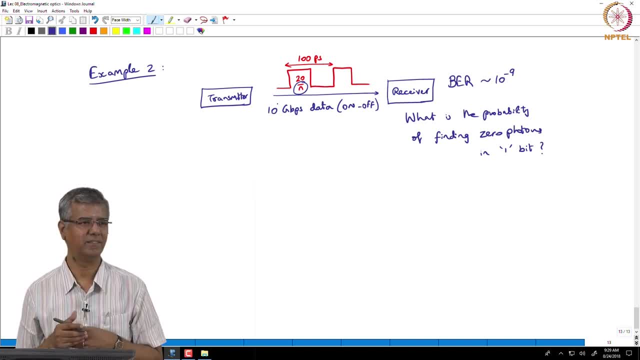 I mean, something is got to be there. So you would say that it is impossible that you will have, you know, 0 photons corresponding to that. but we will look into that little more detail now. Ok, The general misconception about light when we measure light, is that we typically do. 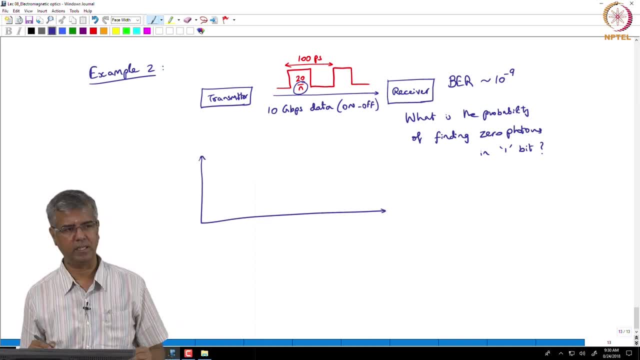 what you do in the lab is actually you measure using a power meter. right, and the power meter essentially shows that it gives the power as a function of time. So over a period of time you say that you are transmitting a mean number of photons in that 1 bit at the receiver and 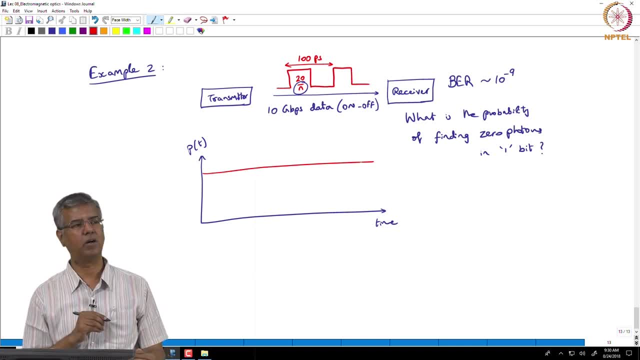 you can say: the intensity is constant, right, So that is what you are seeing. But what is the time scale with which the power meter is providing its value, doing the measurement? it is typically. you know it has got some integration time and all that millisecond is typically typical time. 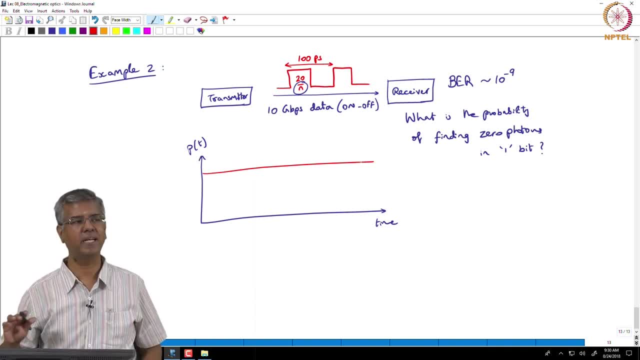 scale that you have right In the millisecond time scale, everything looks constant. You get the perfect reading, you know 3.14, and so you put then the reading 3.14 milliwatt. But does that mean that you have a uniform stream of photons hitting that power meter? 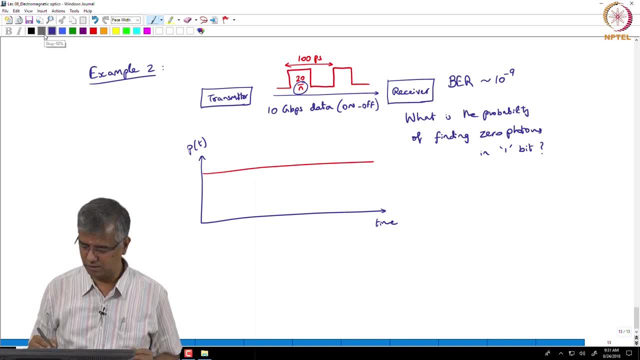 Actually not, because if you look at, if you actually do this, you know, if you look at, you know if you have a smaller sections in time, especially if you go down to kind of the time scales that we were projecting in the previous case, you will find that ok in this time slot. 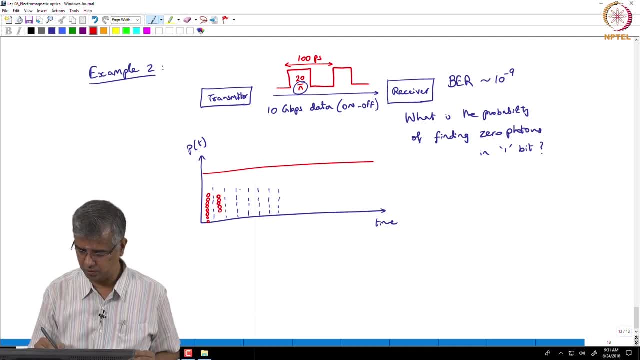 so many photons came in this time slot. so many photons came in this time slot, maybe a few more photons came, And maybe you would have a time slot where only a few photons came, And then another time slot where there is a much, many more number of time slot that came, and so on. right, You get the picture. 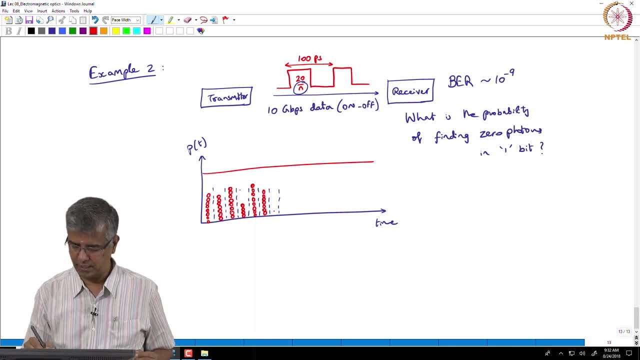 So what I am trying to illustrate here is that, even though your power may show up, as you know, uniform in milliseconds- 17.51 milliwatt, 18.51 milliwatt time scales- If you go down to nanosecond, picosecond time scales- what you may actually 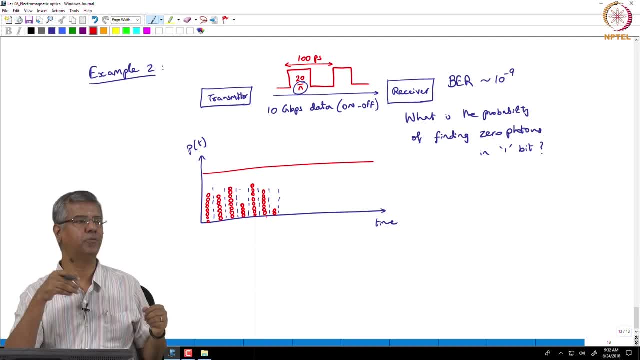 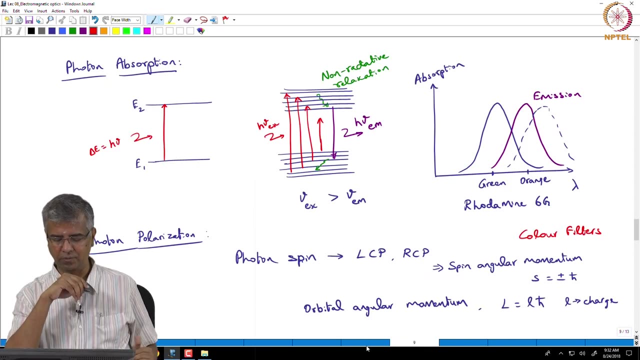 find is that it is not uniform, really ok. Why is this the case? I will just give you a clue. at this point we do not have a lot of what do you call lot of data points to say why, but I will just give you a clue. here We were looking at this picture of photon. 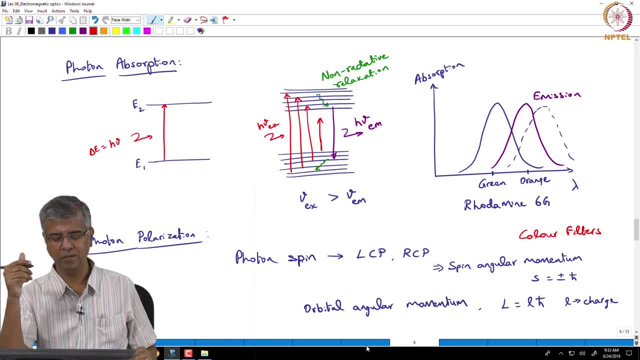 absorption and emission, and when we talked about a particular thing over here. there is a lifetime over here, right? So there is a lifetime that it spends in the upper energy level before it comes down to the lower energy level. Now that lifetime for Rodaman 6G is about 10 nanoseconds. ok, In fact, we were trying to. 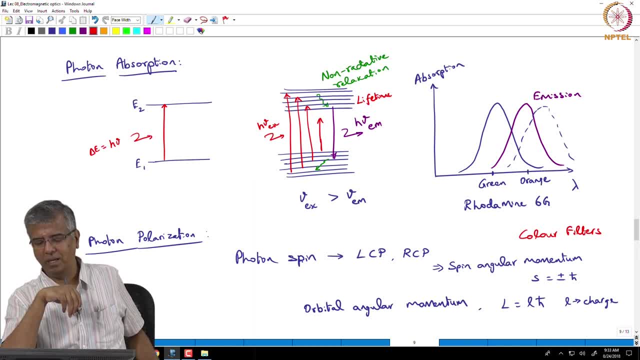 do a demo where we can measure this lifetime, but unfortunately that did not work out, because the we cannot generate pulses that are much faster than 10 nanoseconds with the equipment that we have with us, But nevertheless the lifetime is approximately 10 nanoseconds. 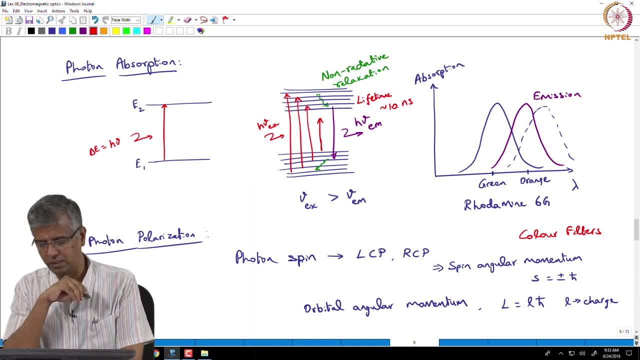 right for Rodaman 6G. So what does this lifetime mean? Does it mean that every electron that goes to the upper energy level, it spends exactly the 10 nanoseconds and then after that it emits? Not really It. actually it is a probabilistic event. I was mentioning that this absorption is a 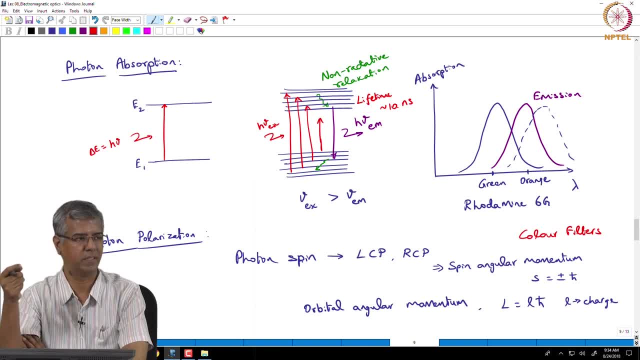 probabilistic event. the emission also is a probabilistic event. So what is the lifetime? So what is the lifetime? So what is the lifetime? So you can only tell in terms of some mean probability right over some mean time, over which this 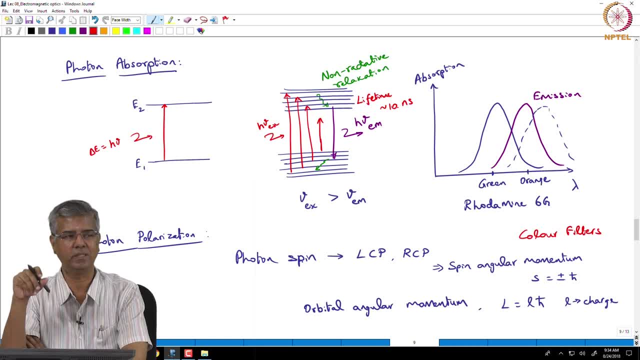 emission happens. In fact, this lifetime is defined as, if you look at, if you send a pulse of light, for the excitation that you will have an emission corresponding to that, which will be high initially because a large number of electrons are at the higher energy level, and then some of those 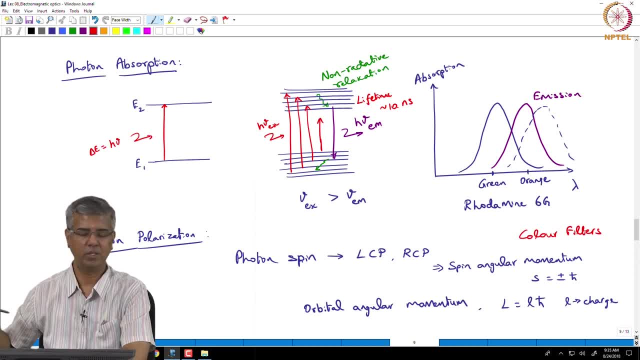 electrons are starting to emit, So your fluorescence. if you look at the fluorescence as a function of time, you will see that it is actually coming down in an exponential manner because there is a finite reservoir that is built in. with every photon that is emitted, that reservoir is getting emptied. So you know, when you look at the rate at which the power 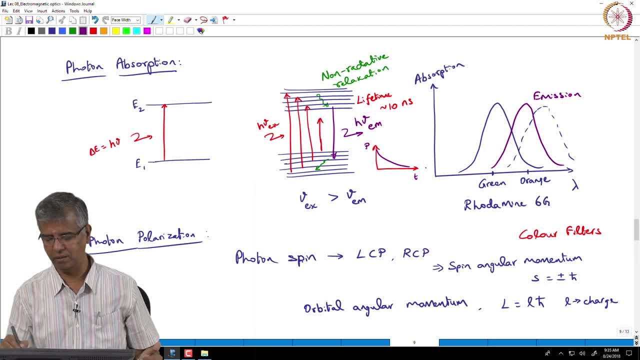 is emitted. as a function of time, it will come down exponentially, and the 1 over E point is what you figure out is the fluorescence lifetime. ok, So what that says is that the photons are emitted continuously. well, it is of course quantized wave packets that are emitted, but they are. 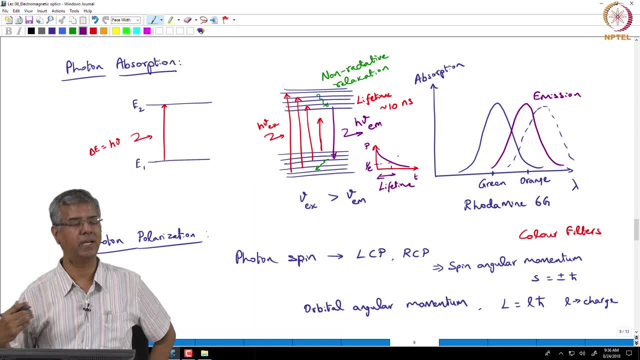 emitted at different times. So you cannot control this is a quantum event. you cannot control this. to say that it emits only at that, this particular picosecond right, So it actually. you can track the envelope of that, but you cannot tell this photon is going to come at this particular time. 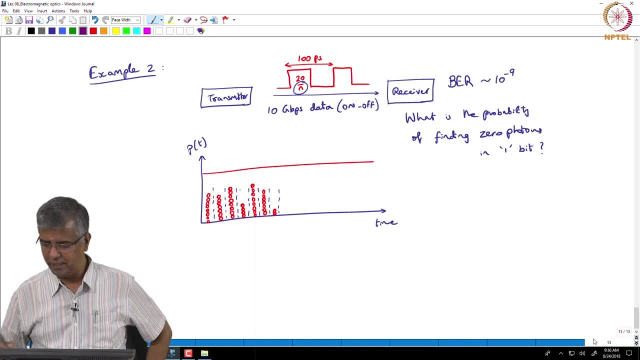 So we are just building on that. in saying that, when you think about light emission, we think about light that is falling on me, you are detecting that in an integrated manner. you are not seeing photon by photon If you go down to a picosecond time scale. 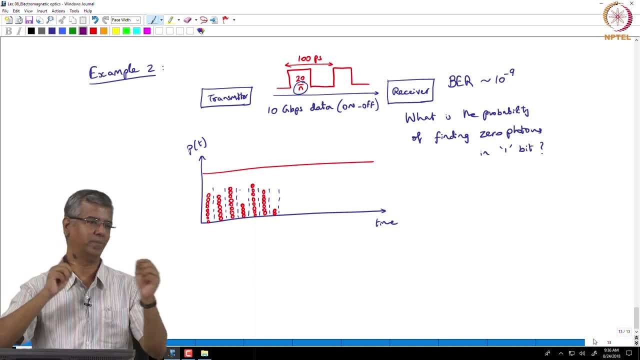 you would probably see that this photons are coming at some random manner. random it is emitted and some random time scale, right, So they are not coming uniformly. ok, that is the point. So your arrival statistics at the receiver: ok, that actually follows what is called a Poisson distribution. So, since these photons are 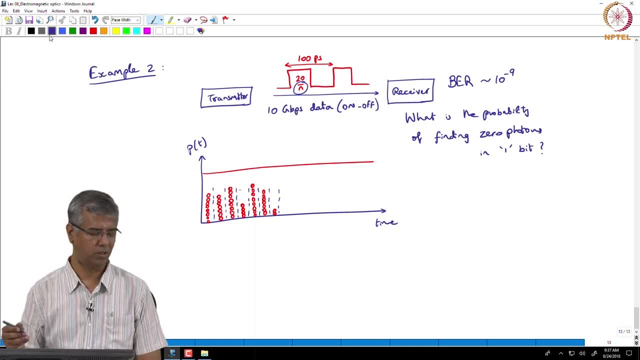 independently emitted. ok, the arrival status you have what is called Poisson arrival statistics. ok, and it is actually not too difficult to derive this formula for Poisson arrival statistics. It is one of the example problems that is given in your text book but you can show that probability of finding some n photons. 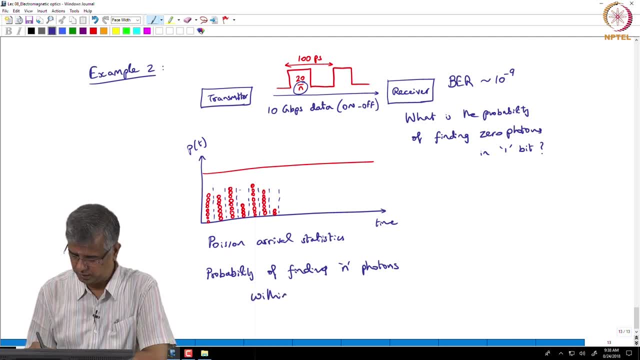 within ion governments Ok. interval in any given time interval you denote as P of n. In this case, what you have done is you have sent a mean number of photons, n bar, ok. So if you take the mean of all these small, 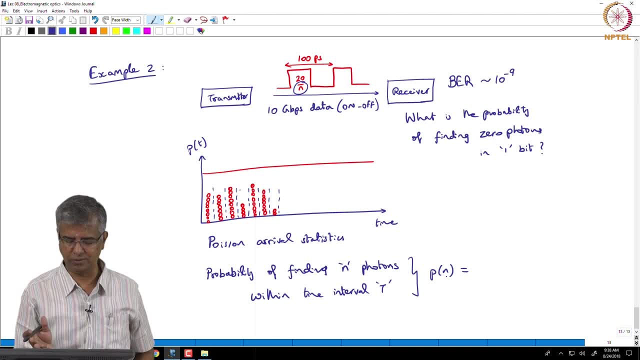 circles that I have drawn here, that would probably correspond to mean of 6 across all these things. So let us say you have sent 6 photons. what is the probability of finding one photon in one of these time slots? right, that is what we are trying. 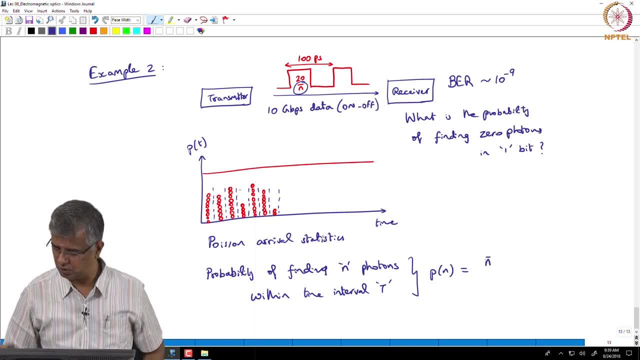 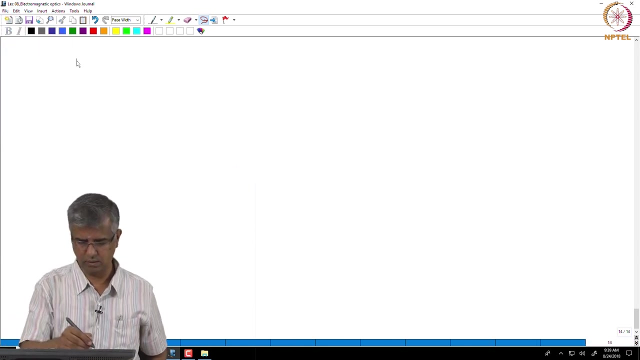 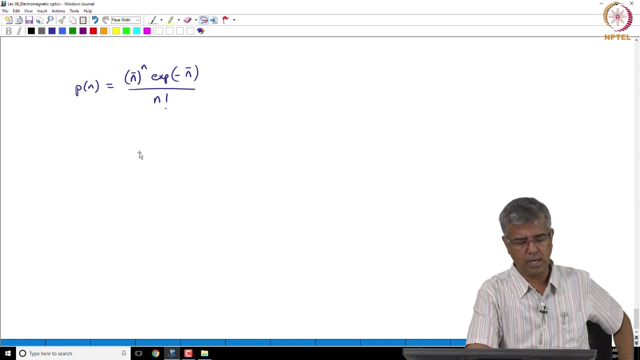 And that, for Poisson statistics, works out to be n bar to the power of n exponential of minus n bar divided by n factorial. ok, So this is basically the Poisson statistics. ok, So let me actually select this and I will just. ok, So that is the probability that 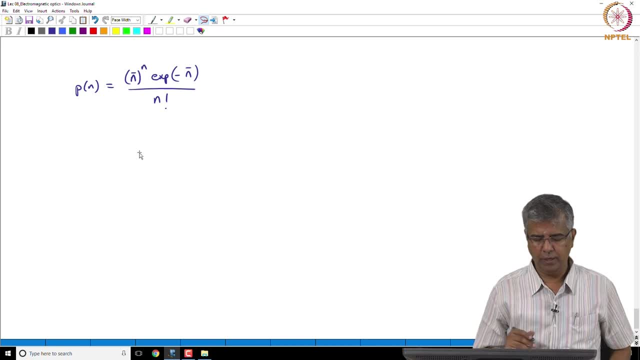 we have. ok, Now, if I try to plot this, then we may actually get a clear picture of what this means, what this Poisson arrival statistics mean, right? So here I have n and I am plotting P of n, 1 and let us say: plot this in log scale, So 0.1,, 0.01 and so on, and n, let us say 0,, 5,, 10,, 15 and. 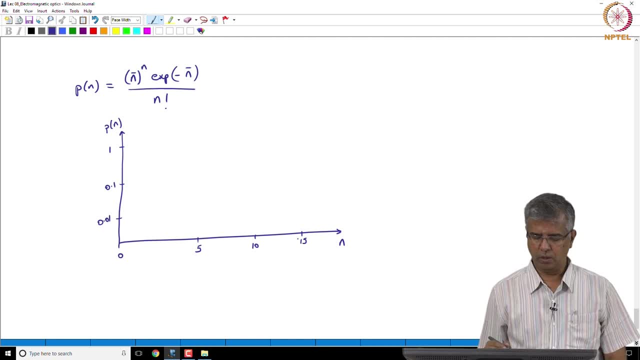 so on. ok, Now let us plot this function for n bar of 0.1. ok, So, So average within an interval is 0.1.. So you would say: how can I express it as a fraction? Well you, 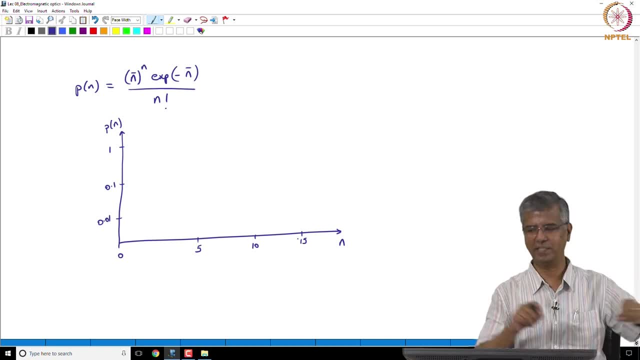 cannot like tear the photon and say, ok, this much is going here, that much is going there. no, it is not like that. You are basically saying that the probability of finding a photon over 10 consecutive time scales, that is, time intervals, you know, is 1.. So it could. 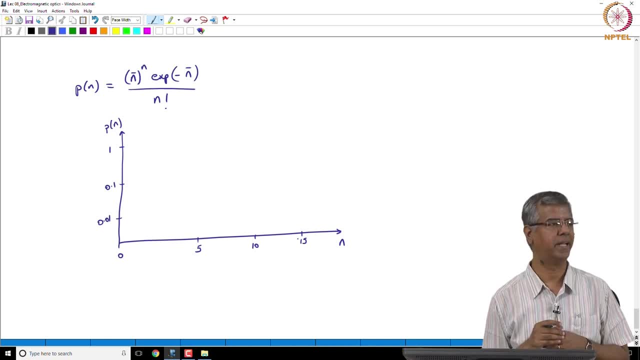 appear in any one of those 10 time slots. ok, So that is what n bar of 0.1 mean. But, interestingly, if you plot this, you would find that you have a very good probability that you will find no photons in a given time slot. 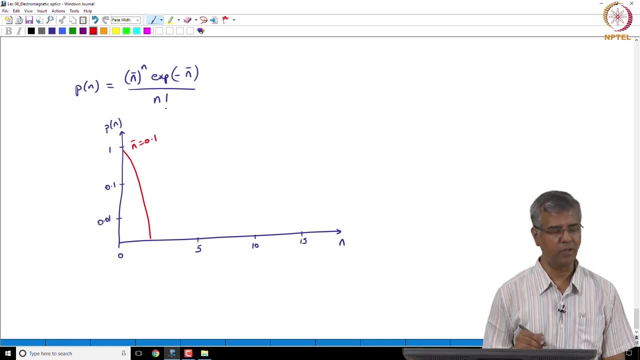 right. There is still a very good probability that you will find- I mean, you will find- one photon. there is a finite probability that you will find one photon in that time slot. or you could even have two photons in a time slot. There is a finite probability. 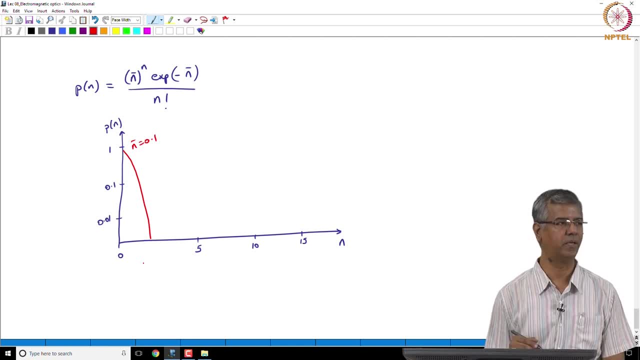 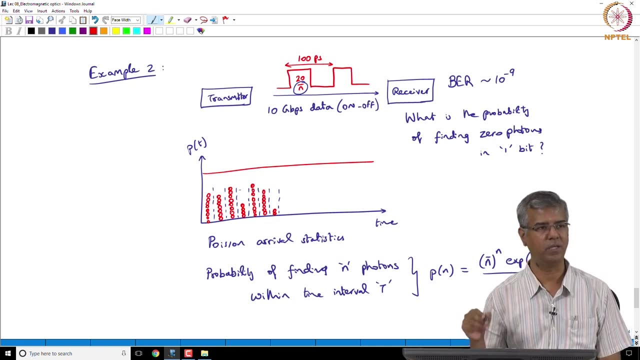 the, however small the probability is. there is a probability. Why are we tracking this? Because our problem requires us to find 0 photons when you have a 1 bit. So you there, you have n bar of 20 and you are asked to figure out what is the probability that you 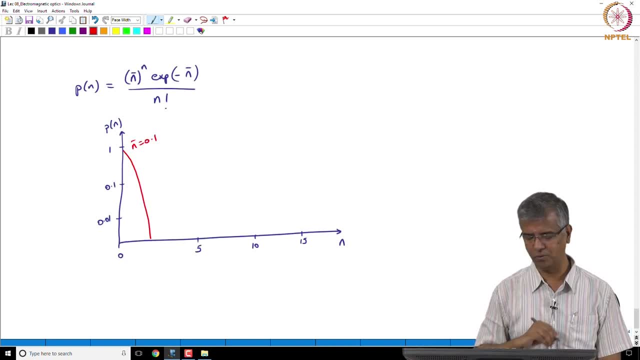 find 0,, 0 photons in the in the time slot. So if we work further, ok, Let me choose a different color. and if you, if I say n bar of 1, that is going to look like this. right, I am just giving you a general perspective. do not pay too much attention. 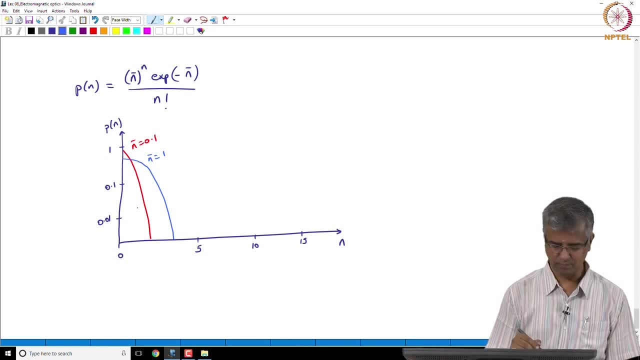 to the specific numbers here, and if I go to n bar of 5,, ok, It is going to look like that. and similarly, if I go to n bar of 10 and and if I still go on to to What we are looking for for, n bar of 20 would have probably looked like this. So, of course, 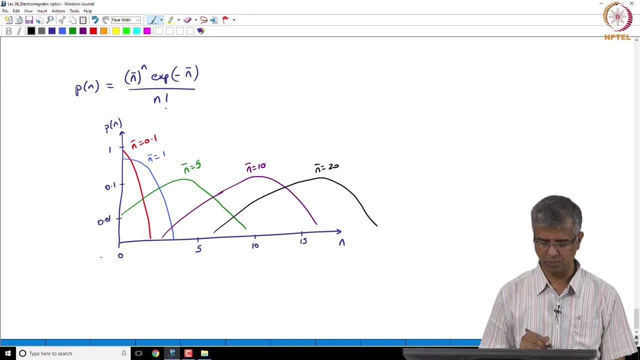 we have a scale here, the y scale, where we have only up to 0.01,. but if you just extrapolate over here, you will find that it goes to a fairly low value. So what we are actually trying to do is that we are actually trying to do, is that we are actually trying to do? 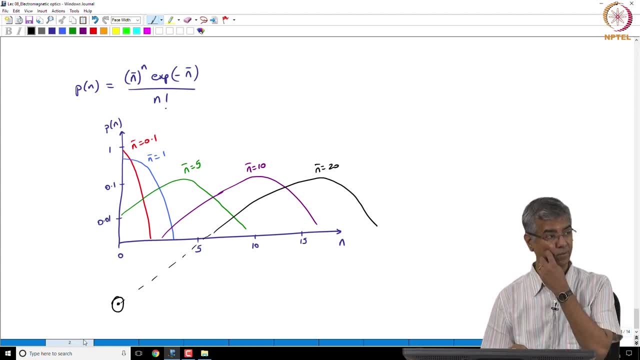 is that we are actually trying to find out. is this point over here? So you have n bar of 20 right that has been sent by the transmitter. that is the average that you have sent, but you could have a probability that 0 bits are there in that time slot. ok, You have a finite. 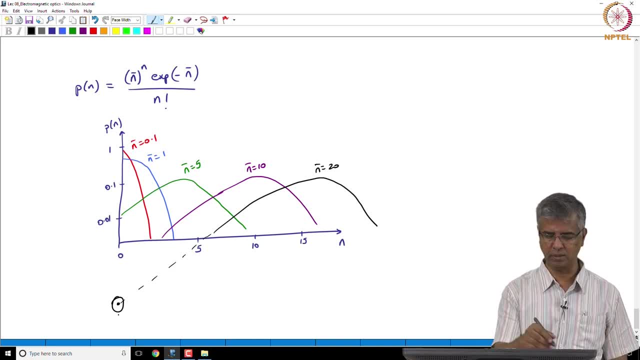 probability. If you work out the though this, this expression, over here, what you will find that this probability corresponds to 2 into 10 power minus 9, ok, So, 2 times out of 10 power 9 bits, right, So that is, that is a billion bits. ok, So. 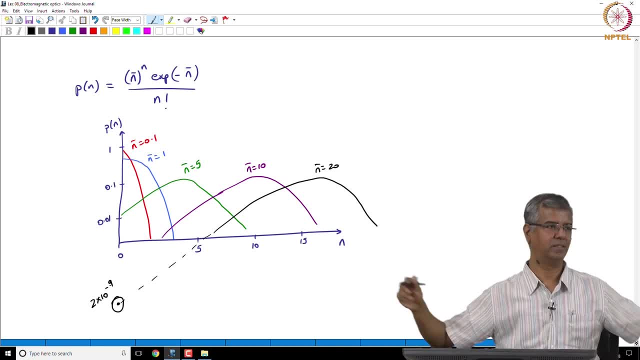 if you have, if you have collected 10 power, 9 bits, then then you may find that there are 2 bits where this, this sort of Occurrence, is happening. ok, That seems like a very small number, but it is still significant in communications. because of what? Because you are transmitting at 10 gigabits per second. 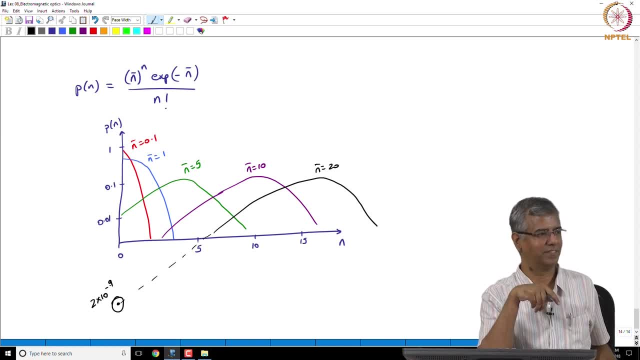 So within a second, you might actually see 2 of these events, ok, So, so, so that that that is the thing, but but, of course, like I say it is, it is relevant because of the high speed at which we are transmitting information, but but the key point is, you cannot say that. 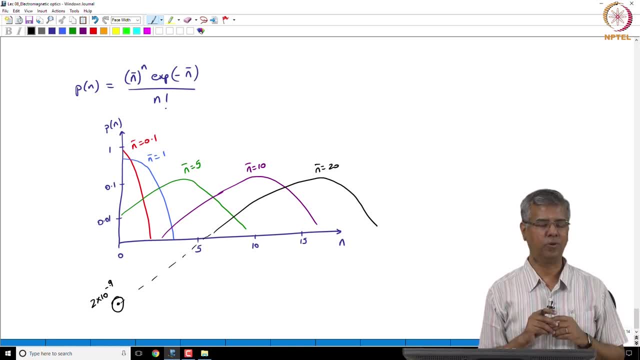 I am transmitting 10 photons in this slot and expect that you know. all these slots are having only 10 photons. It could be 10, it could be 9,, it could be 8, it could be 12, it could be 20,, it could be 0. Each of these have a finite probability, ok, So when we 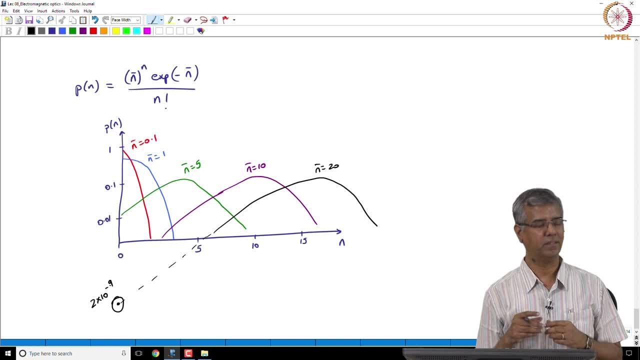 are talking about Photon streams. this is what this is one of the important concepts that we need to understand: that that you cannot control, you cannot time the photons so precise, precisely, ok, Just one quick thing before I end this, if I just go on to looking at for a Poisson distribution. 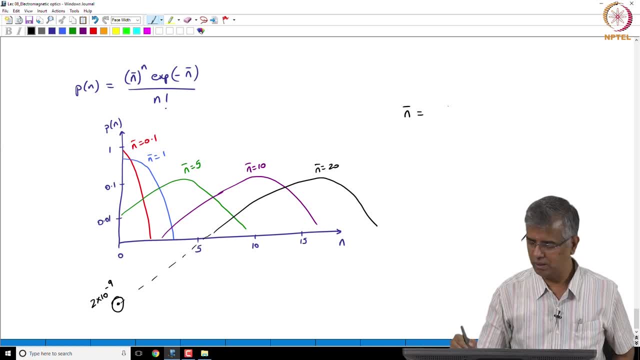 if you look at the mean number of photons That would correspond to, you have all these possibilities that it could be 0 or all the way to infinity, but the probability of those are are weighted So n into p of n is the mean. 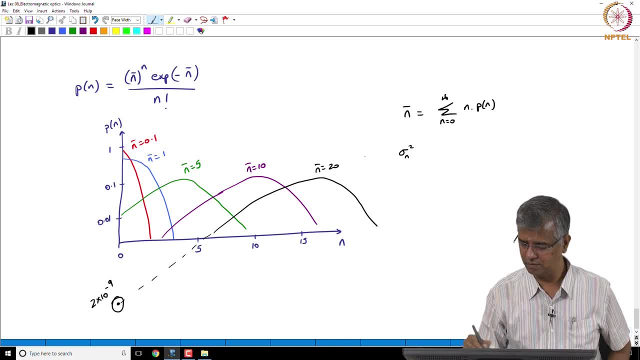 and, more importantly, if you look at the variance, So this is the mean and this is the variance Variance for a Poisson distribution works out as infinity n minus n bar the whole square p of n, and if you compute that interestingly, what you find is that corresponds to n bar itself. so the mean and the variance of a 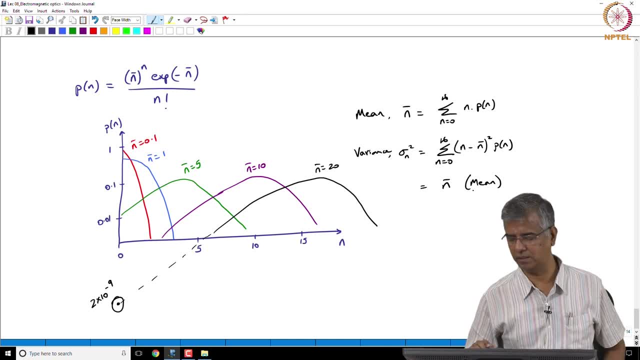 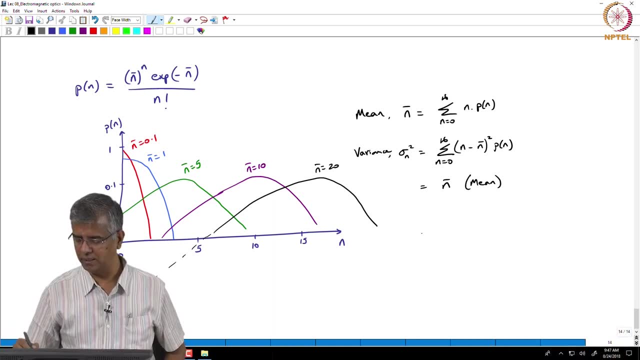 Poisson distribution are the same. ok, So that is an important, you know aspect of Poisson and the consequence of that is when you are looking at the signal to noise ratio, most of the communication applications, most of the practical applications of light, we are interested. 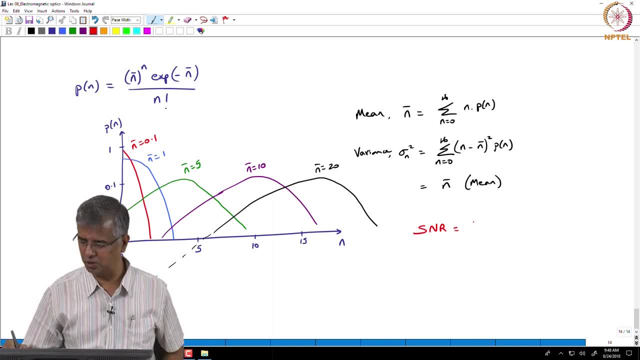 in the signal to noise ratio. So the signal to noise ratio, calculated in terms of photons, it corresponds to the square of the mean over the variance, which is the noise right. So in this case that since you have a mean square divided by the variance which is the mean, So 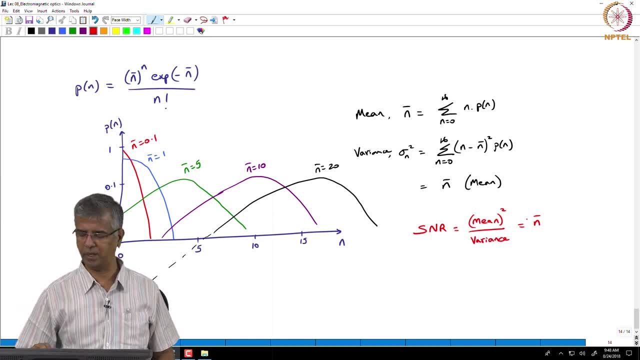 you. your signal to noise ratio goes as mean on the photon. So if you want to improve your signal to noise ratio, you want to have a larger mean number of photons, right? That is what it means. as for, say, a communication application concern, Of course, 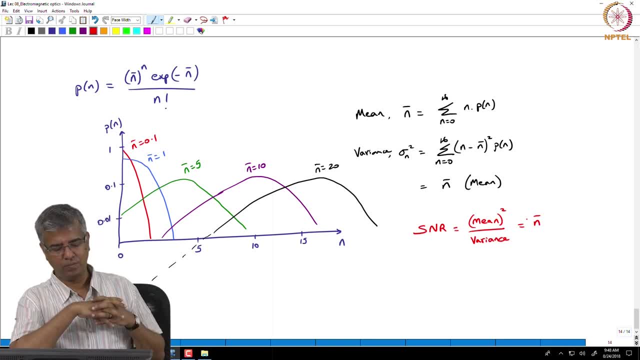 that means that you want to flood your- you know your- time slots with photons. but it is not as simple as that, because in practical systems we find that beyond a certain number of photons, if you put into the medium So you can start touction process, the medium starts behaving in a non-linear fashion. 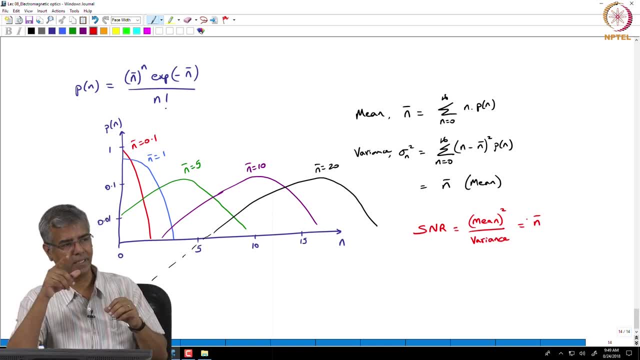 ok, That epsilon that we are talking. what the permittivity, which is the response of the medium for a given excitation or given electromagnetic wave. right That response? it is linear up to a certain number of photons. beyond that it is starting to behave non-linearly. So you can. 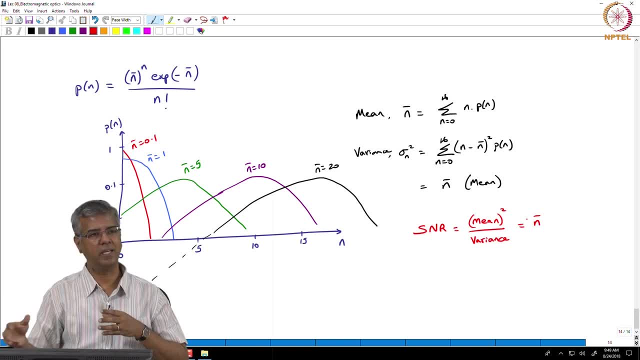 extend this argument, you know, to a very large number of photons, because you know you will start hitting this. nonlinear issues, and that is one of the major research areas in optical communication today. How do you, you know, prevent nonlinearity from happening in the optical communication system and still get very good signal to noise ratio? So we are out of time. 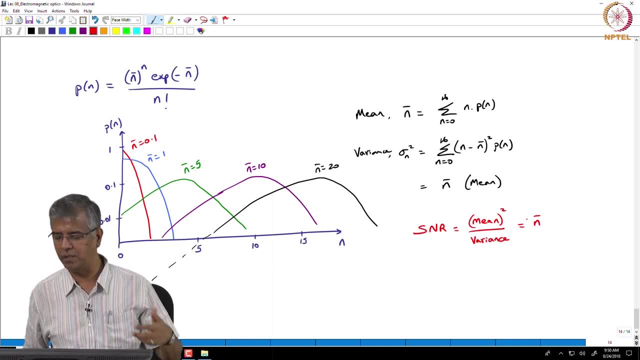 now. So let us stop at this, and what we are going into now is looking more closely at the absorption and emission of photons. How does that happen in different systems? What are the properties of those photons, and so on. So we will going to build towards.